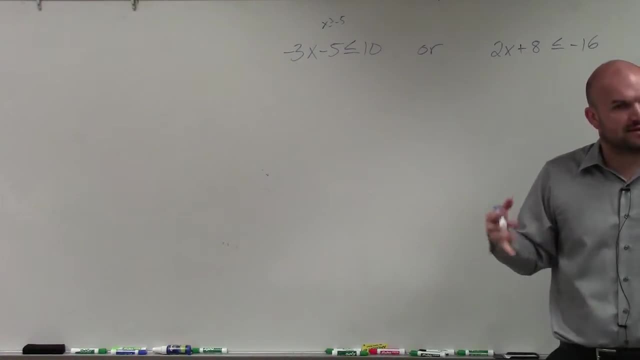 understand that you can break those apart into an and statement, because really we're only dealing with and and or statements, but there's two representations for and, So, when looking at this problem, all we're simply going to do is solve them separately. 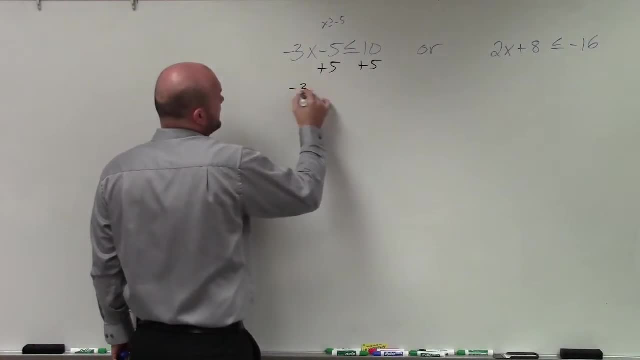 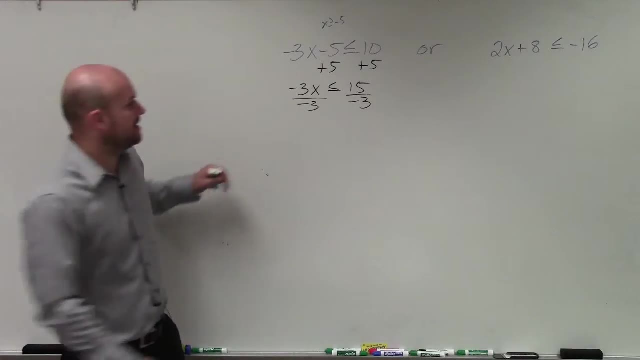 So I'll add five here. Add five Negative three. x is less than or equal to 15.. Divide by negative three. Divide by negative three. Please remember, whenever you multiply or divide by a negative number, x is greater than or equal to negative five. Right, Jacob. 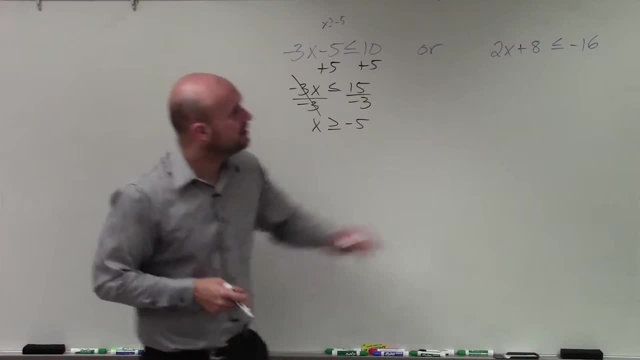 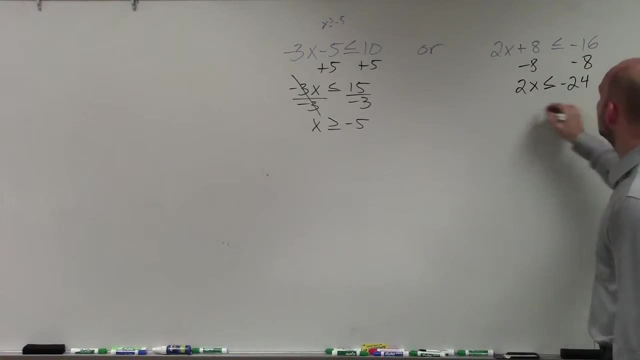 make sure you flip that sign. It's going to happen. I'm telling you Over here we go ahead and solve. So I subtract eight. Subtract eight Two x is less than or equal to a negative 24.. Divide by two. 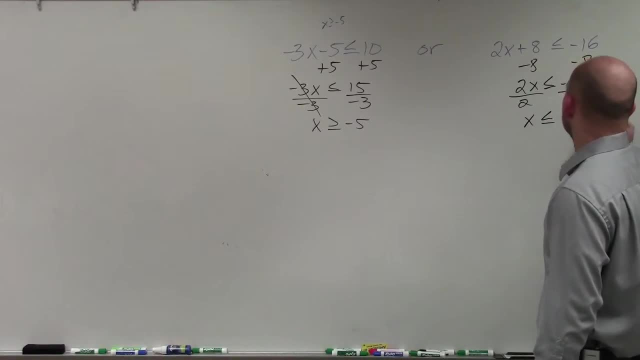 Divide by two, X is less than or equal to a negative 12.. Okay, Notice, on this one I didn't flip the sign. Some people say, oh well, you're dividing, you know, into a negative number. That's okay. But notice what my divisor is Here. it's positive, so I never flip the. 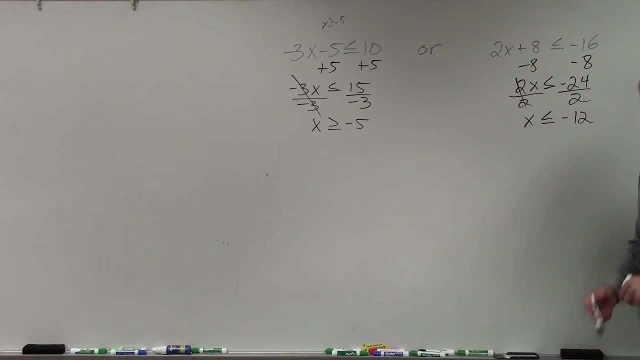 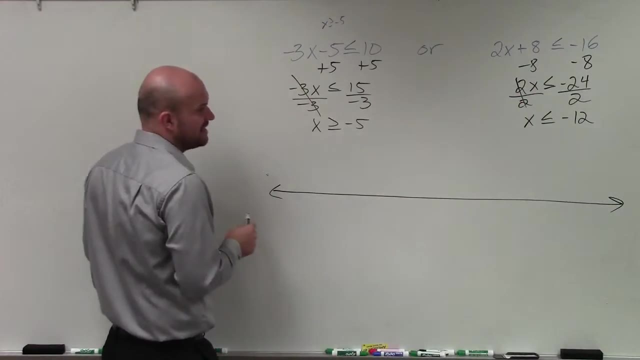 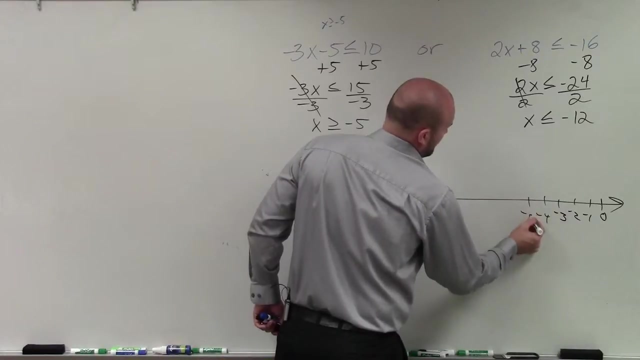 sign Here. my divisor is negative, so that's okay. So I'm going to flip the sign Here. that's why I had to flip the sign. all right, Now we need to create a number line that's going to contain negative five and negative 12. So I put zero over here. negative one: 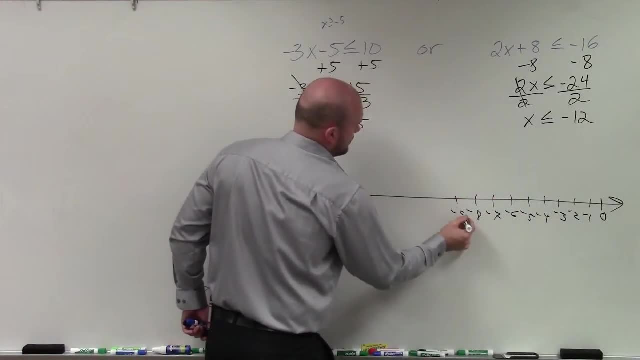 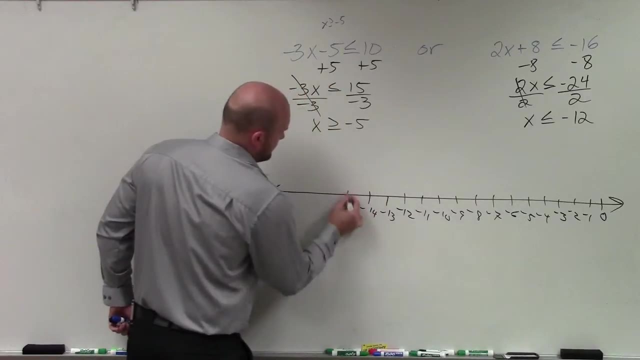 negative: two Speaker: 15 Speaker 16 Speaker 17 Speaker 18 Speaker 21 Speaker 23, Speaker 24, Speaker 27, Speaker 28, Speaker 24, Speaker 28, Speaker 39, Speaker 31,. All right, so again, ladies and gentlemen. 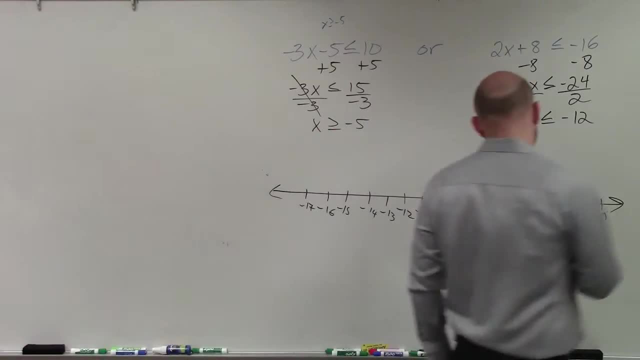 we're going to do what we know how to do. We're going to go to our two points and make dots there. So I have negative 5 and negative 12.. In this case, I'm going to use test points rather than going to the left or to the right. 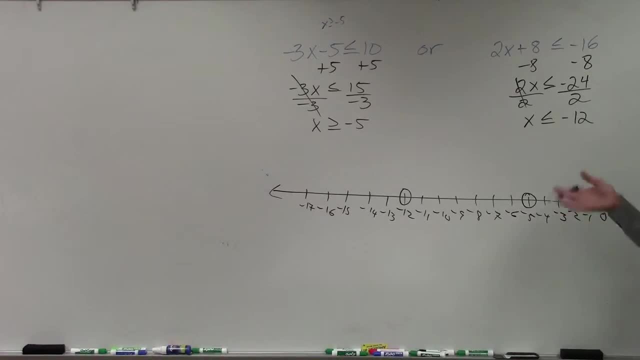 because I think negatives always get people confused, So I'm going to use test points. First of all, though, we don't need to use test points for these, because we can look at the inequality symbol. Are both of these a part of the solution? 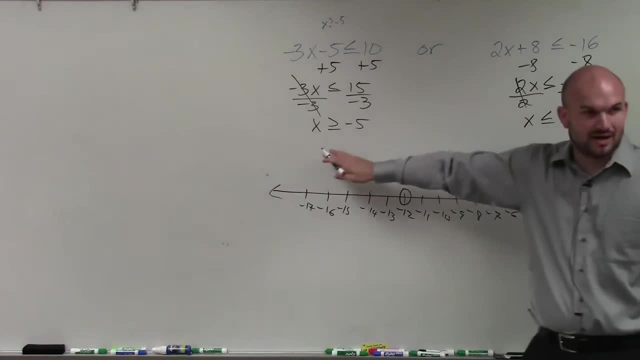 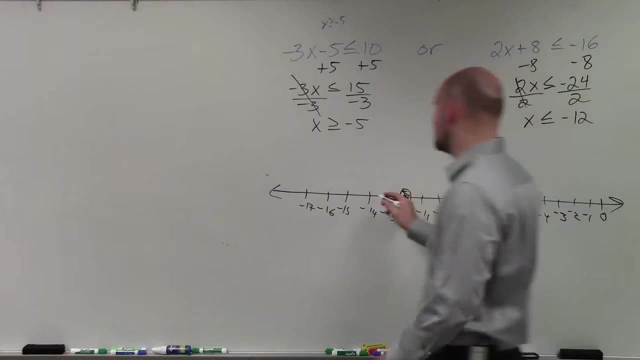 Are they closed or open? Closed because they're equal to, greater than or equal to, or less than or equal to, So we can close them. We can also use test points. Now to use test points again, what I'm looking for. 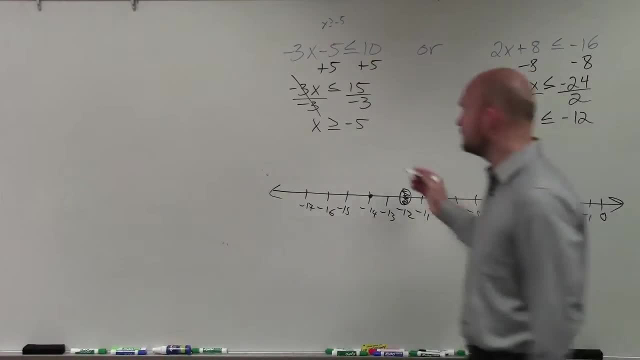 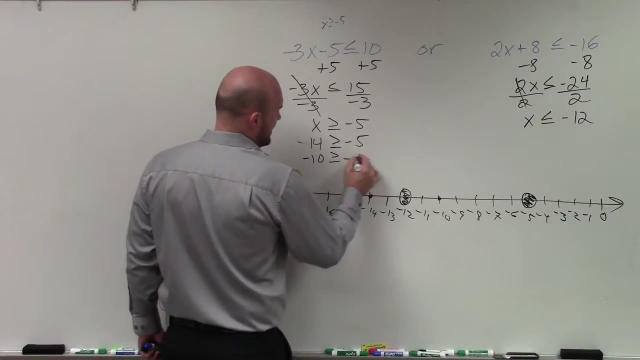 is just picking a point to the left and to the right and plugging that point in for x. So negative 14 is greater or equal to negative 5, or negative 10 is greater or equal to negative 5.. And again one of the statements is going to be true. 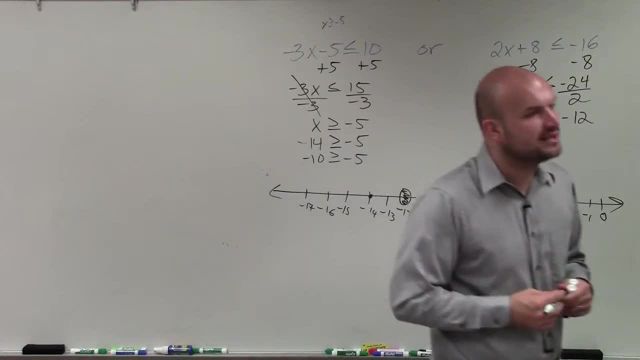 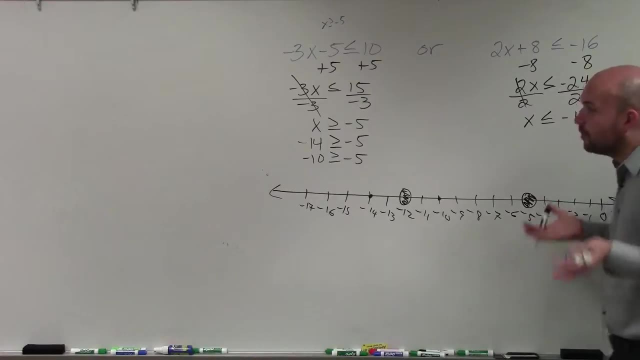 One of the statements is going to be false And please just remember: when thinking about negatives, think of negatives as money you owe somebody. So if you have, how much? what is more, If you owe somebody $14,, do you have more money? 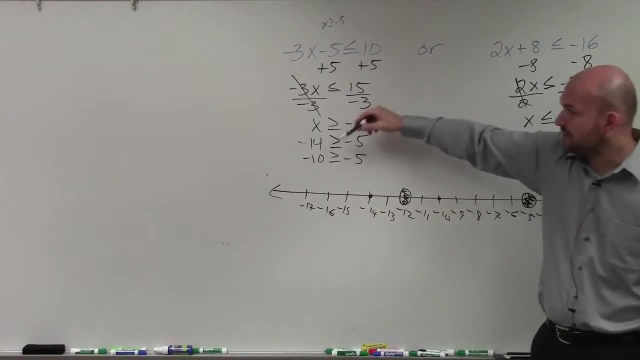 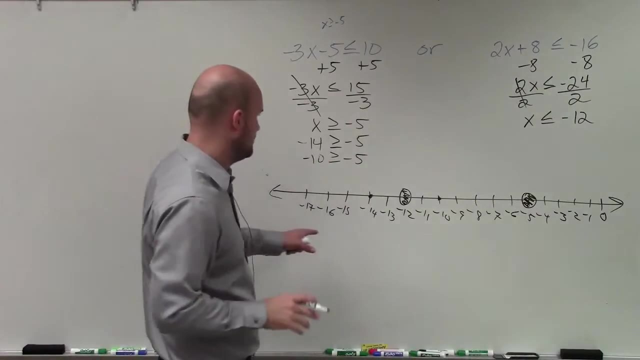 than if you owe them $5? No, If you owe wait a minute, what did I do? You did it with 5, not 12.. Yeah, 12.. Wait, Oh, I did 12, OK Here, sorry about that. 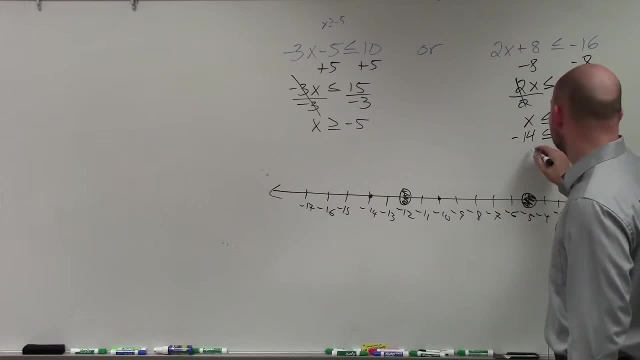 Negative 14 is less than or equal to negative 10.. Negative 12 or negative 10 is less than or equal to negative 12.. So if you owe somebody $14,, do you have more money or less money than if you owe them 12?? 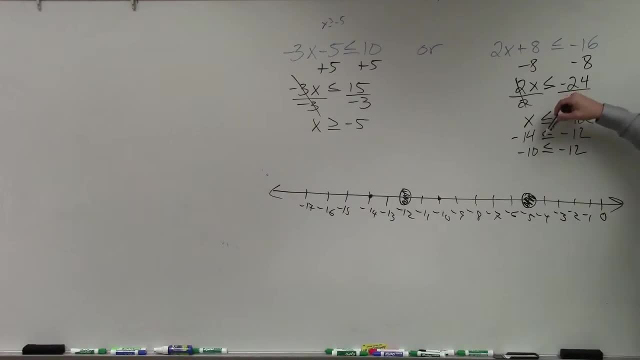 You'd have less money. So is that true or false? That is true: If you owe somebody $14,, you have less money than if you owe them $12.. If you owe them $10,, you do not have less money than if you owe them 12.. 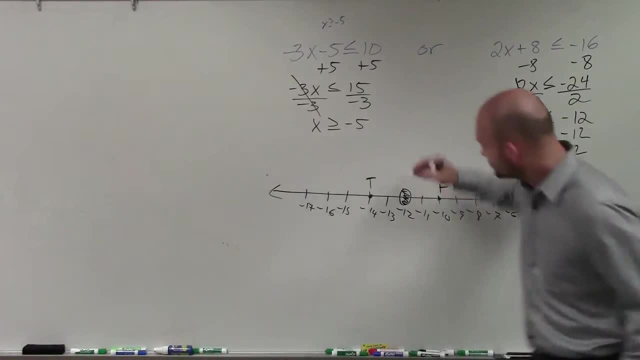 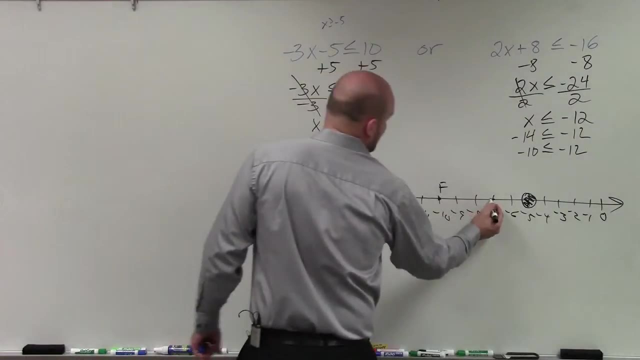 So 14 is true, 10 is false. So therefore my graph is going to go to the left Over here. we'll do our two points. I'll pick 7 and 3.. Negative 7 is greater than or equal to negative 5.. 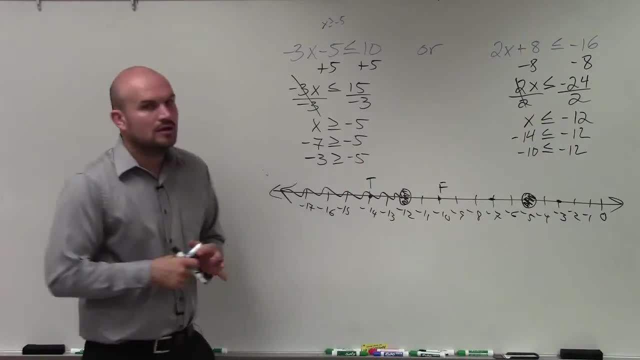 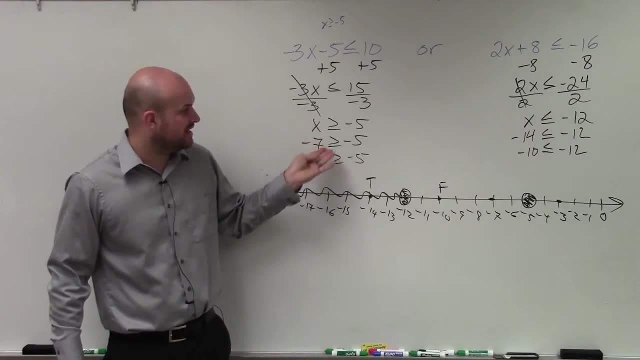 And negative 3 is greater than or equal to negative 5.. Again, what the states is: if you owe somebody $7, do you have more or less money than if you owe them $5?? And obviously you'd have less money if you owed them $7.. 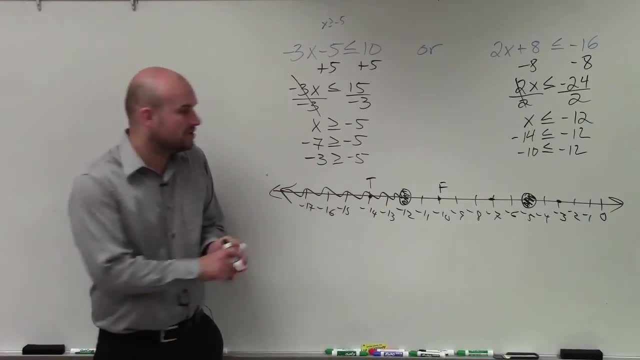 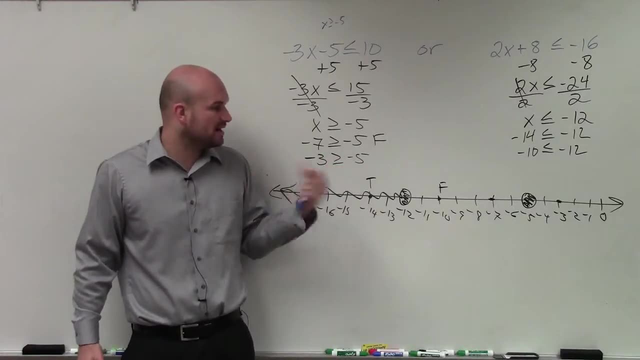 Right, So 7 is not greater than. It's less than. So that's false. But if you owe somebody $3, is that greater than owing them? Do you have more money than if you owed them $5? Yes, So this is true.